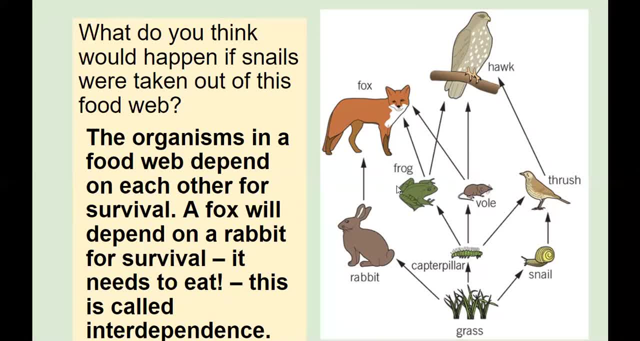 caterpillar will be eaten by the thrush, meaning there's less food for the frog and less food for the vole. If there's less food for the vole and for the frog, then there'll be less food for the fox and the hawk and the rabbit. So they're all dependent on each other and we call this. 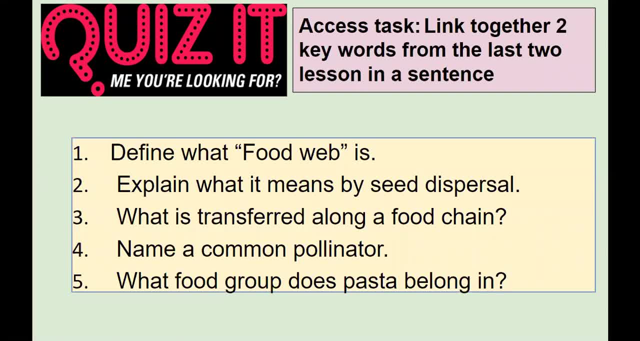 interdependence. Okay, so quick five questions. Define what a food web is. Explain what its means by seed dispersion. What would happen if the snail was eaten by thecoin? And then what would happen to the snake? And if the snail was eaten by the frog? then there's less food for the frog and 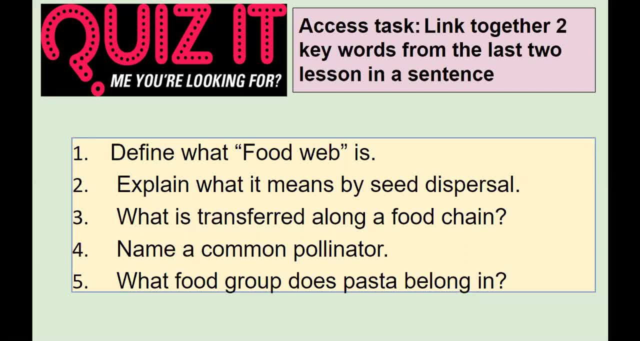 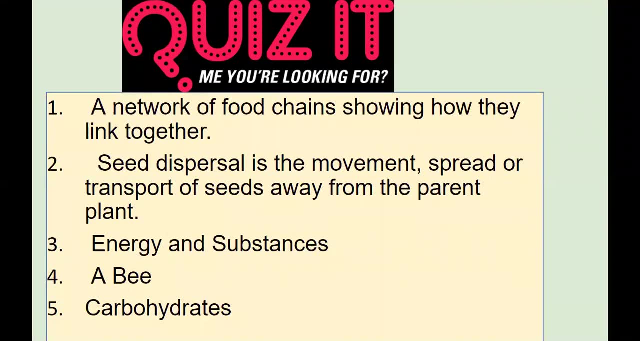 question three: what is transferred along a food chain? question four: name a common pollinator. and question five: what food group does pasta belong into? okay, pause the video and have a go at those questions. okay, so food web is a network of food changing, showing how they link together. seed dispersal is the movement. 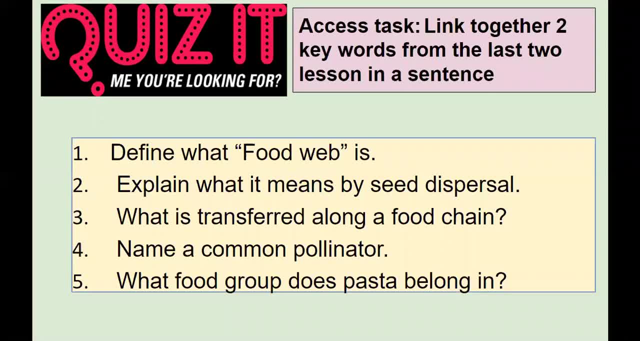 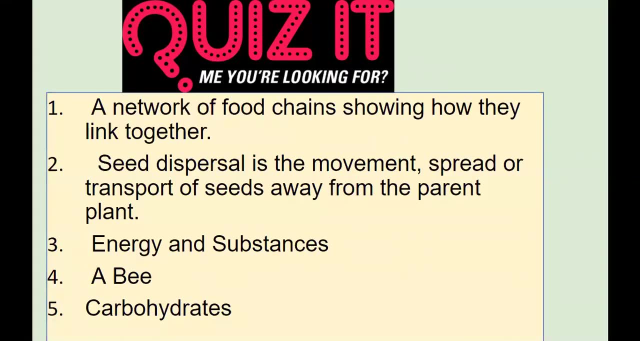 or the spread, or the transport seeds away from the parent plant, what the transfer of energy and substances is. what's transferred along a food chain? a common pollinator is a bee, and pasta belongs to the food group of carbohydrates. give yourself a mark for everyone. you've got right there, okay. 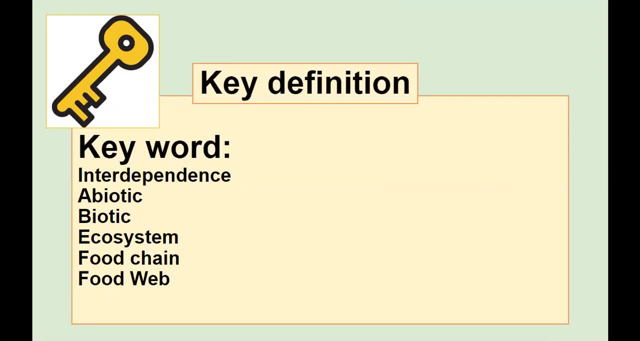 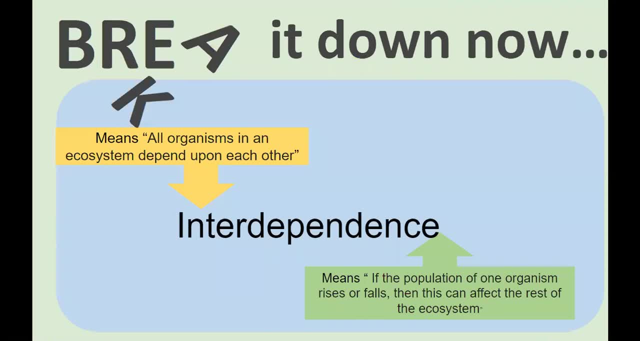 keywords for this lesson, then interdependence, abiotic, biotic ecosystem, food chain and food web. so the word we're going to look at now is interdependence came up on slide one. interdependence means all organisms in an ecosystem depend upon each other, and if you don't remember what ecosystem means, then please do research that one. 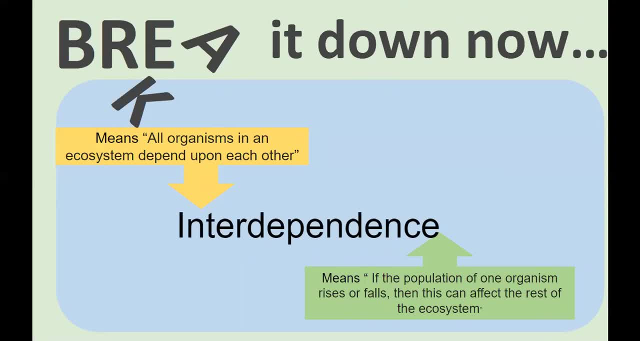 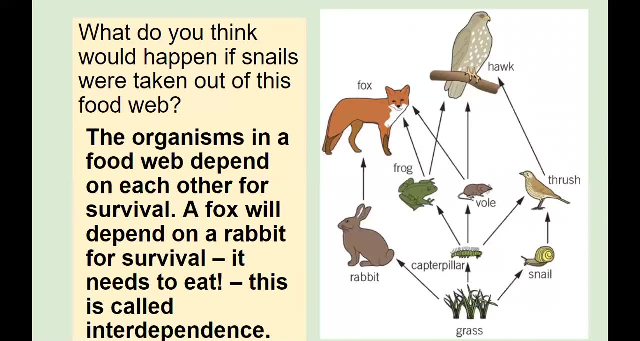 so interdependence also means if the population of one organism rises or falls and this can affect the rest of the ecosystem. so, going back to the snail, if the snail's population was to decrease- and the first would have to depend on the caterpillar for food, and if the caterpillar is being eaten up by 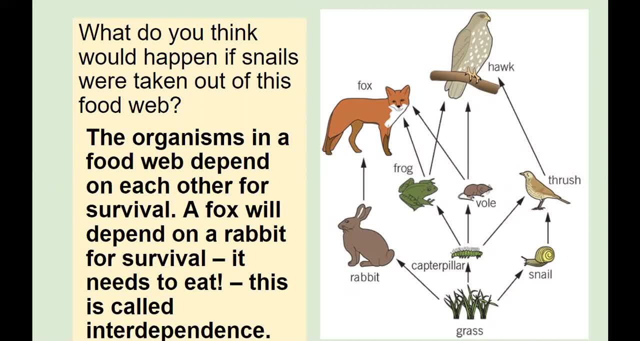 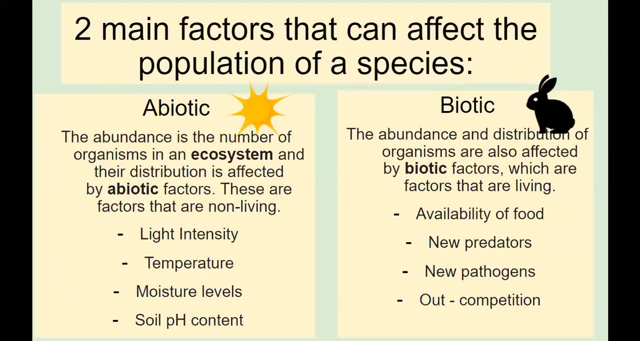 the thrush, there may be less for the frog and for the vole, and that will have an effect on the hawk and the fox and the fox, sorry. okay. so there are two main factors that affect the population of the species and we categorize them in two different categories. so we have abiotic. 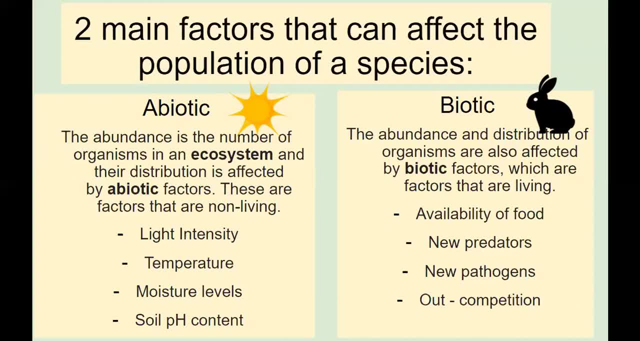 and biotic. so abiotic is a factor that is non-living, so an abiotic is the abundance, is the number of organisms in an ecosystem, and their distribution is affected by abiotic factors. these are non-living things, so this could be a light intensity, the amount of sunlight available, the temperature, so how hot, or 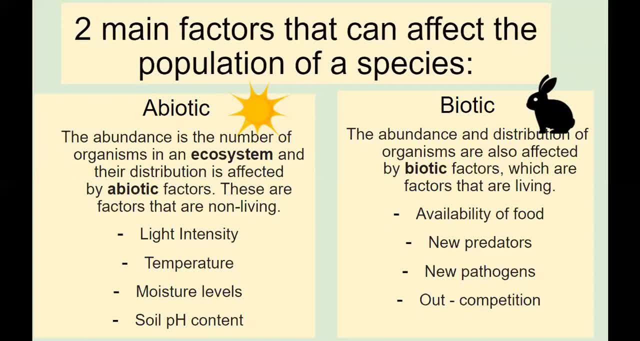 cold. something is moisture levels, so whether there's a lot of water in the air, and the soil pH content. so when we look at pH we think about how acidic or alkaline the soil is and obviously this can have a effect on the growth of plants. so the other category is biotics: the abundance and distribution of 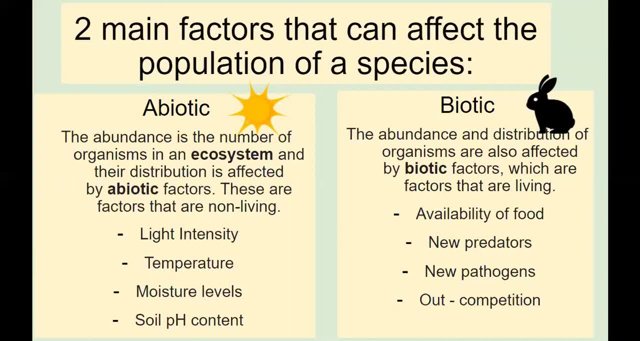 organisms are also affected by biotic factors and these factors are living, so the available food. so whether there's a lot of food to eat- new predators. so if you were to introduce a big old wolf to an ecosystem and it's gonna eat a lot of the prey. 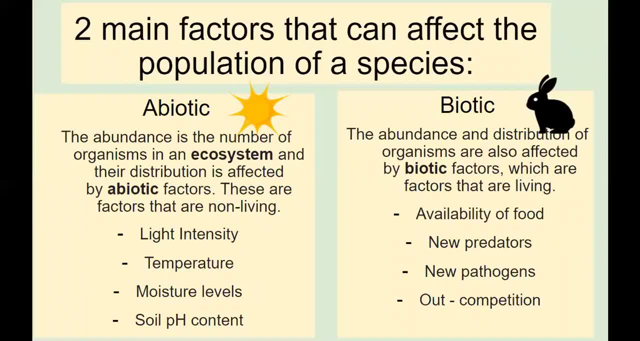 there new pathogens. this is things like bacteria, viruses, protists and fungal. the new for system or out competition, so whether there's competition with the different species in that environment. so it might be worth to do a quick table and give examples of abiotic. biotic factors affect the population and distribution. 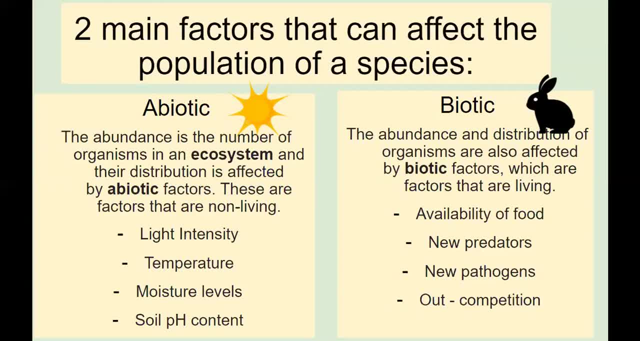 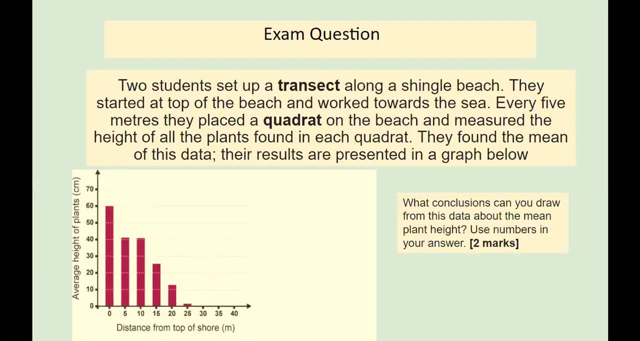 the species within an ecosystem. Okay, an exam question. then. The two students set up a transect along a single beach. They started at the top of the beach and worked towards the sea. Every five meters they placed a quadrat on the beach and measured the height of all the plants found in. 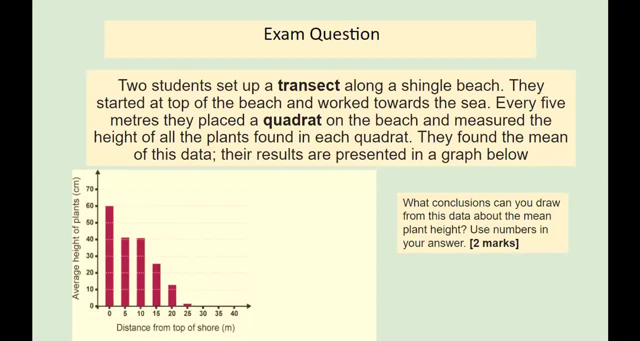 each quadrat, They found the mean of this data. The results are presented in a graph below. So, as you can see, you have the average height of plants, centimeters, versus the distance from the top of the shore, and there is a distinct pattern occurring within the distance from the top of. 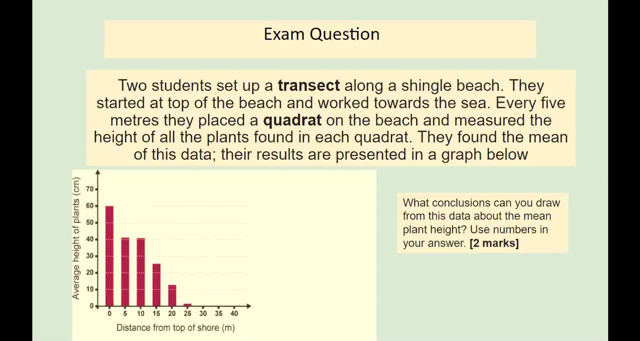 the shore versus the height. So what conclusion can you draw from this data about the mean plant height? Use numbers in your answers. So this is worth two marks. So you would be commenting on what you can see is happening in this graph. You then add validity to your answer by adding: 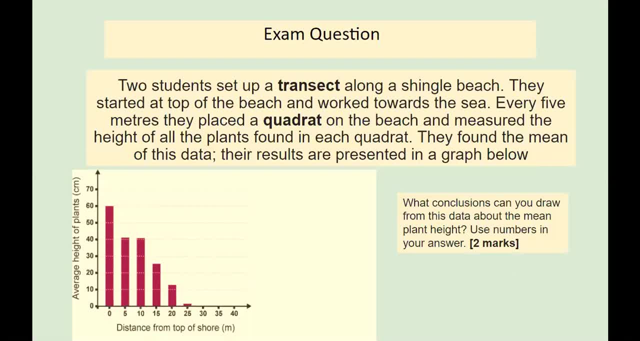 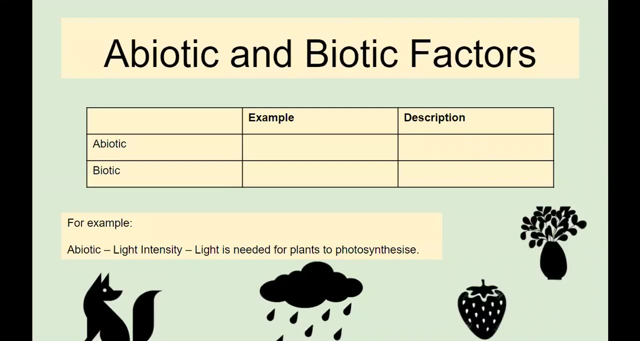 numbers in your answer. So you could say: at zero meters from the shore versus 25 meters from the shore, there is a watch. Is there a decline, an increase? no difference. You need to be able to have a look at that. Okay, so doing an abiotic and biotic factor So you can give an example of an abiotic factor. So 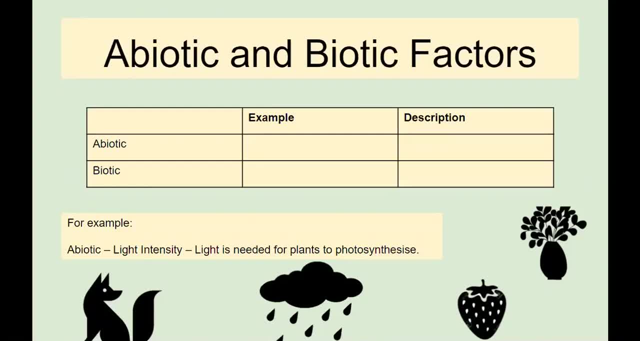 this could be anything from the ones we've seen before, versus the biotic factor, and then you're asked to describe it For example. an example of abiotic would be light intensity, So the amount of light is needed for plants to photosynthesize. So if you haven't got enough light, 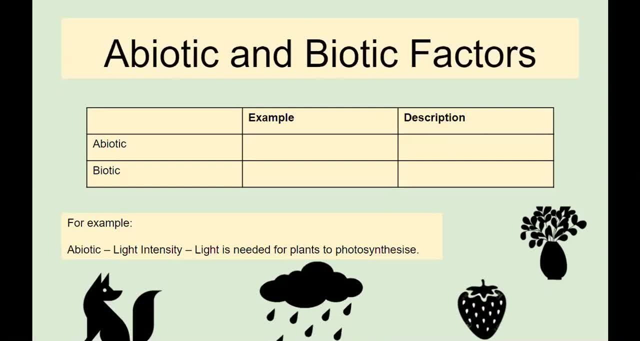 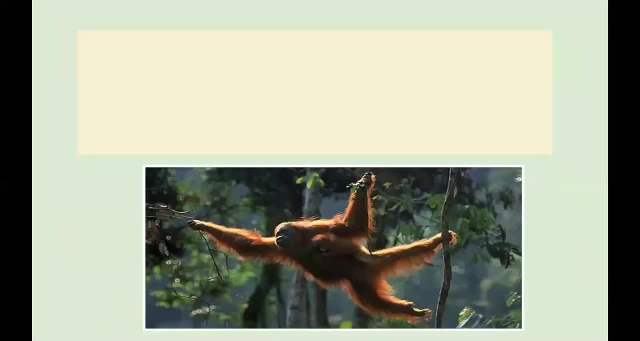 you can use a biotic factor. So if you haven't got enough light, you can use a biotic factor And plants will not be able to photosynthesize, so light intensity. as it's not living, is an abiotic example of something that can have an effect on the ecosystem. Okay, so a nice picture of an. 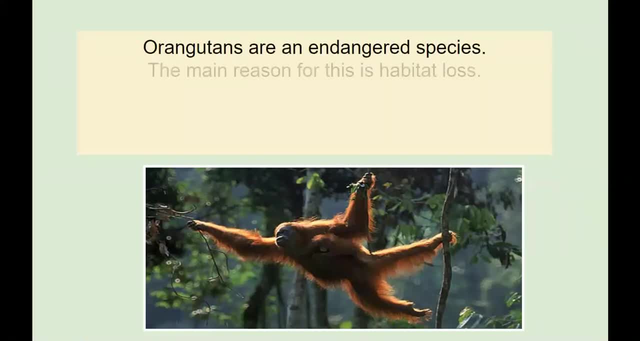 orangutan here. Did you know that orangutans are an endangered species? The main reason for this is because of habitat loss. So even without human interferences, ecosystems are constantly changing. They usually go in peaks and troughs and can change constantly. the factors are continually fluctuating, so this could be the amount. 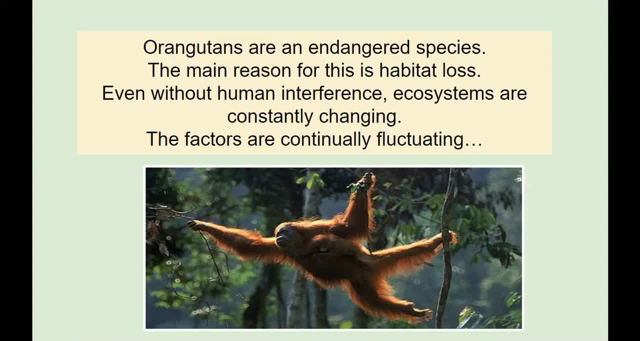 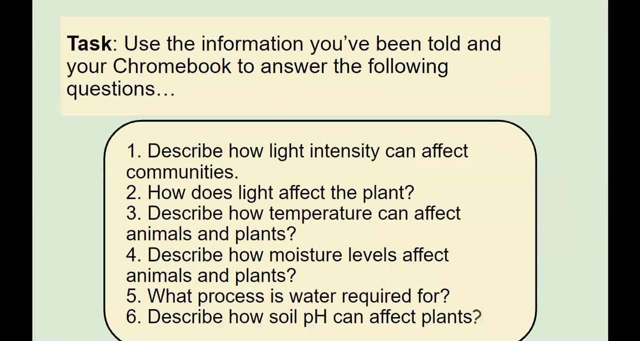 of food resources available. this could be an abiotic reason, with plant growth, not enough light intensity or carbon dioxide present in the atmosphere. can be many different reasons, but if you want to research that, then you can do okay. so, using the information you've been told and Chromebooks, can you answer the 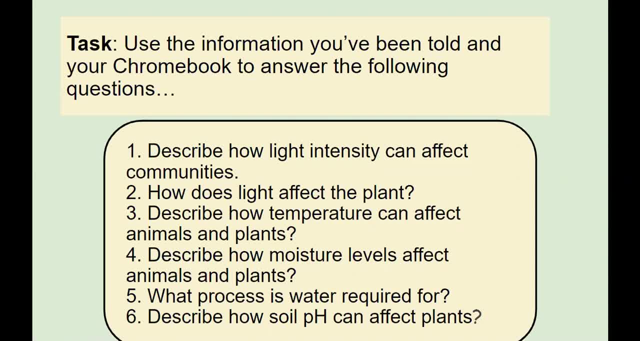 following questions: question 1: describe how light intensity can affect communities. question 2: how does light affect them? question 3 describe how temperature can affect animals and plants. question 4 describe how moisture levels affect animals in class. and question 5: what processes water required for. questions 6 describe how soil pH can affect plants. so quick hint. 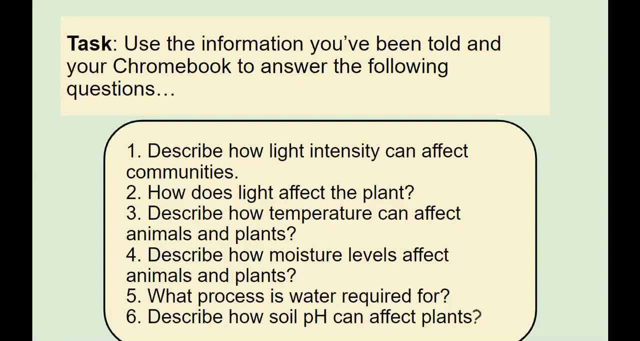 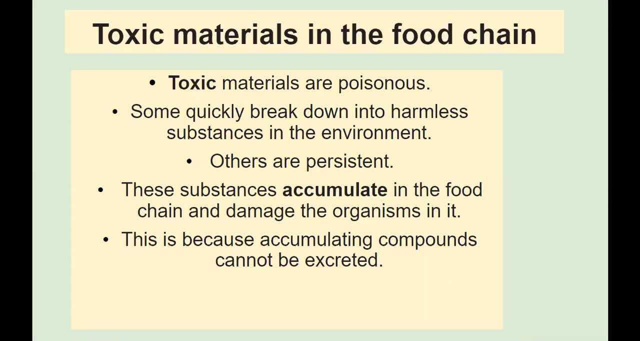 there pH, meaning how acid, acidic or alkaline the ph of the soil is. so, as well as abiotic and biotic factors having an influence in an ecosystem and food chain, there's also toxic materials that can be found in a food chain. when we say toxic, we mean toxic. 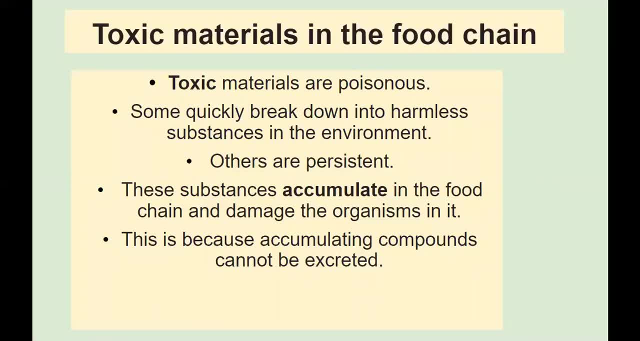 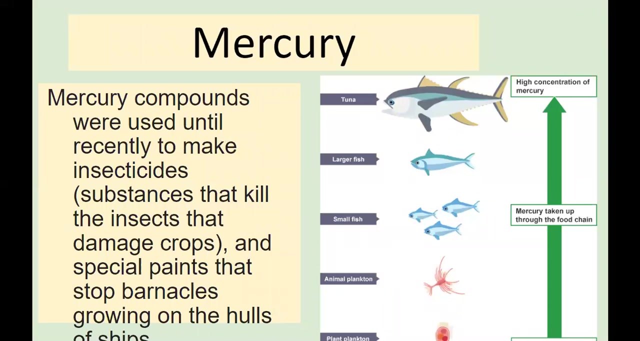 materials meaning poisonous. some quickly break down into harmless substances in the environment and can become quite detrimental, so others are more persistent. these substances, over time, can accumulate in the food chain and damage the organisms within them. this is because accumulating compounds cannot be excreted, so an example of this would be the concentration of mercury within a. 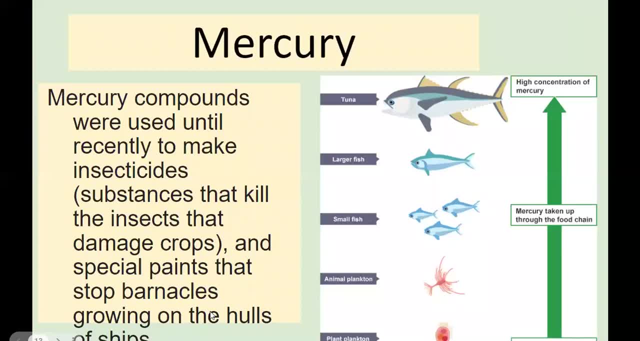 sea. so mercury compounds are usually used- sorry, to make insecticides, which are substances that kill the the the to reduce the amount of insects that can damage the crops. so what they did was they put lots of mercury to reduce the amount of insects on their crops. it's also used for a special paint that. 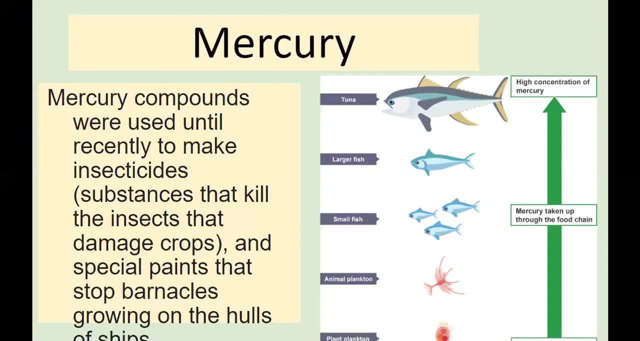 stopped barnacles growing on the holes of ships and what it did was to the fish. as the rate of concentration of mercury increased, the amount of tuna, larger fish, smaller fish, animal plankton and plankton plant plankton decreased. so if the mercury is reintested, the mercury is 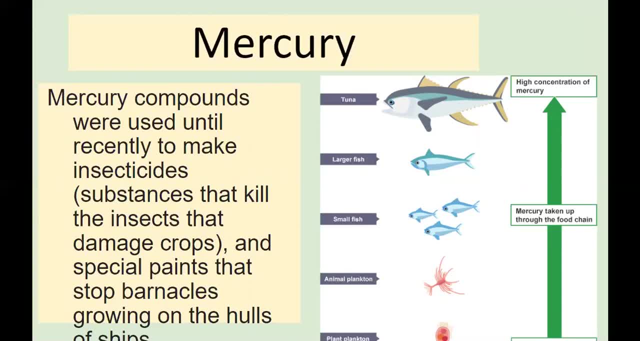 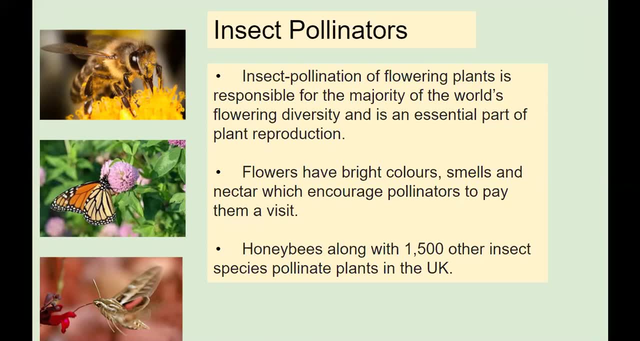 taken up through the food chain and it's going to be absorbed by every animal or plant on that food chain. so that's what we mean by toxic materials within the ecosystem. okay, so moving on to insect pollinators, so we've got some nice pictures here of a common insect. 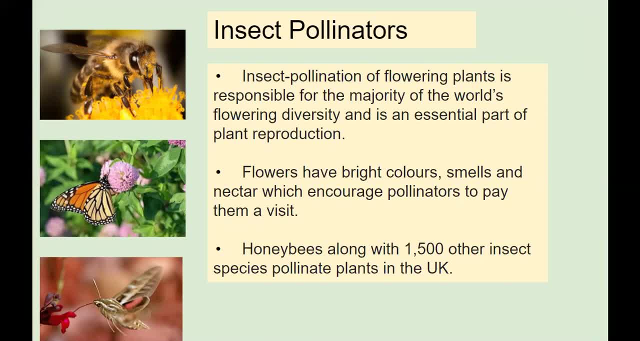 pollinator, meaning the bee. so insect pollination of flowering plants is- bear with me- a sec is responsible- responsible for the majority of the world's flowering plants and the majority of the world's flowering diversity, and is an essential part of plant reproduction. you don't know what. 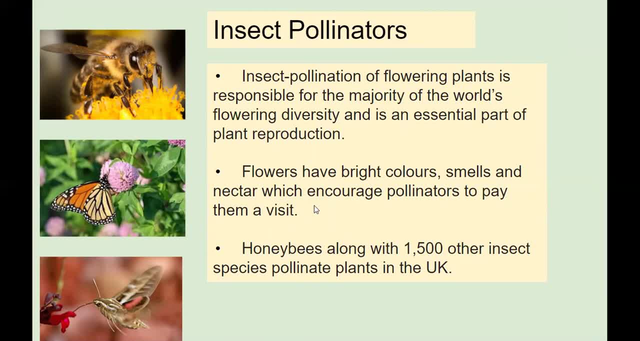 diversity is. you need to be researching it. diverse meaning it's got lots of different flowers, different colors, different species of flowers. to have a diverse ecosystem would mean a lot of differences. the flowers have bright colors, they've got nice smells and they have encouraging nectars, which means that the pollinators are attracted to pay them a visit. 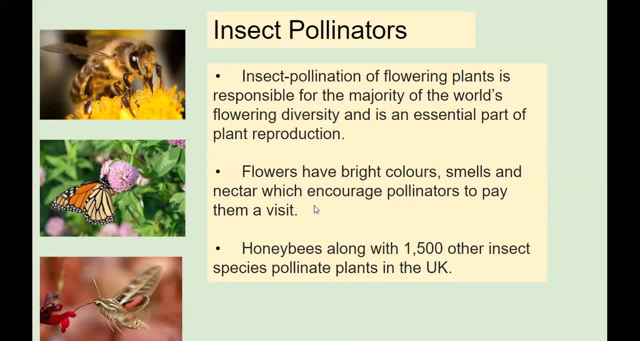 and what this means is that they pollinate the various different plants within that proximity. so quick fact: honeybees, along with 1500 other insect species, pollinate plants in the uk and it might be nice for you to do a little poster on the various different insect pollination of plants.